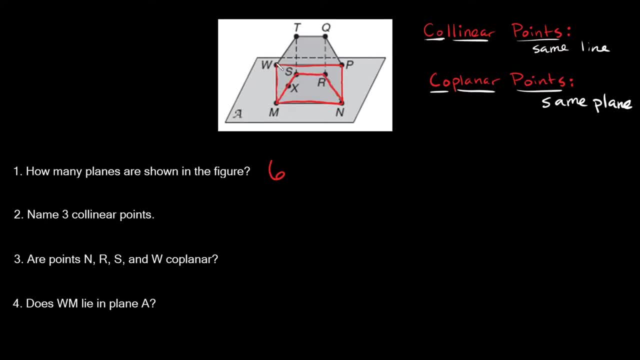 side of the box, that one down there. Okay, we also have this side of the box right here, The right here, on the left right. So we have this left side of the box right there and we also have this other, the right side of the box right. So those are four sides total so far. Okay, don't. 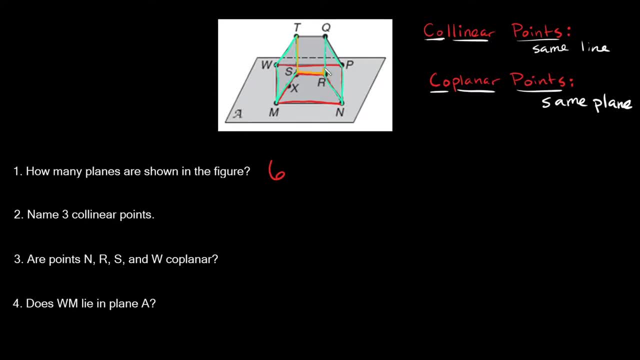 forget about the back of the box, right, Right back there, and then the only part we're missing is the top of the box. So the top of the box would be this one right here. Okay, so, as you can see, we have six surfaces or surfaces, So we have six surfaces. So we have six surfaces. So we have six. 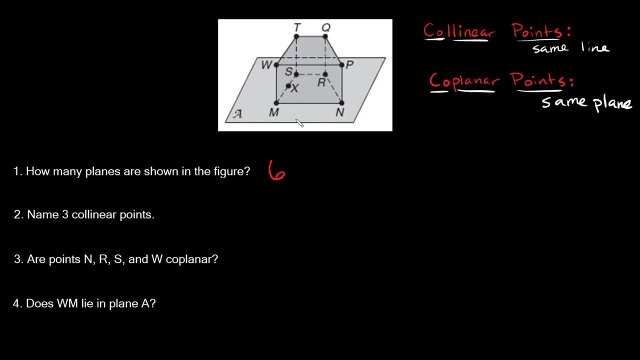 planes to this figure, right to this box. All right, so now let's jump to number two. So it says: name three collinear points. Okay, so remember, these are points that are on the same line. Okay, so three points that are on the same line. well, the only part that happens is right over here, right, m, x and 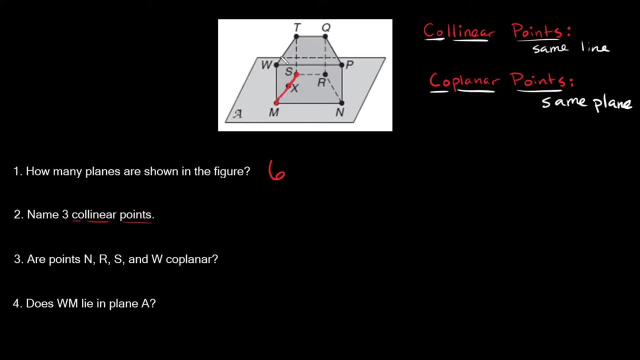 s. This line right here is the only line on this whole figure where there's three points right. Every other single line only Has two points, right. You could literally pick any single random one. So like here we have p and n, right. So there's only two points on this line. All right, what about this line over here? Well, 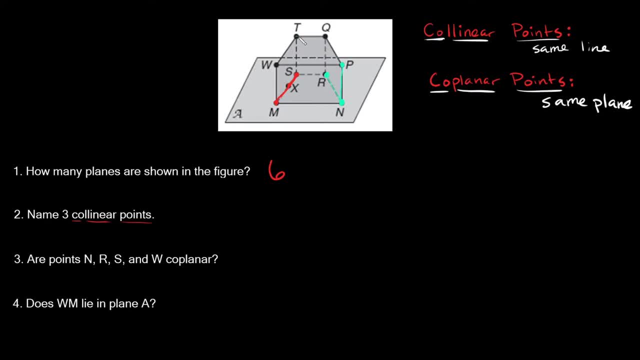 again, there's only two points right: n and r. Okay, what about this line? Well, again, there's only two points right: t and q. All right, so this is the only place where there's three points right, So m, x and s. Name: three collinear points: m, x and s. 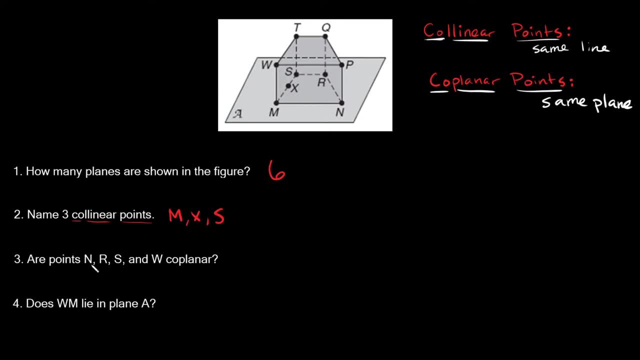 All right, now let's go through this. Let's go to number three. So this one asks: are points n r, s and w co-planar? Okay, so it's asking if all these points right here, n r, s and w, are on the same plane. All right, well, let's see where. 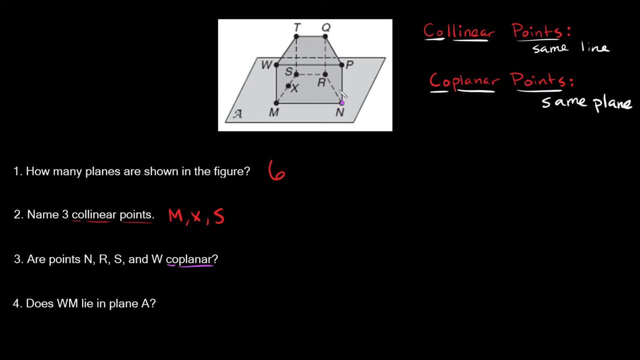 these are n, r and s. n is right there, r and s- Okay. so these three points right here are on the bottom part of the box, right? They're right here. They're on the bottom part of the box, All right. so where's w? Well, w's up here, Okay. so is w on the same side of the box as n, r and s? No, it's not. 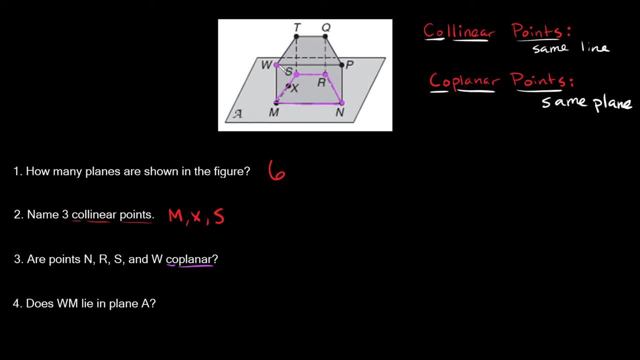 right, Because n, r and s they're on the bottom side of the box and w's on the top corner of the box. All right, so they're not on the same plane. All right, so are points n, r, s and w co-planar. 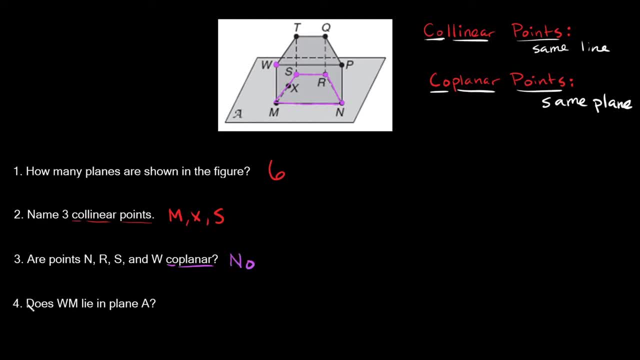 Hell, no, All right. now number four: Does line w m lie in plane a? All right, so first of all, w m, line w m: is this one right here? Right, that's line w m and plane a: is this plane right here? Okay, it's basically on the same side. Think of this as the. 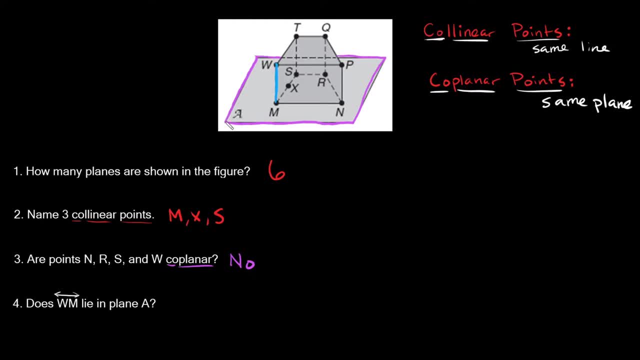 table. Okay, the box is sitting on top of the table. Okay, so this table right here is right underneath the bottom of the box right here. And the question is asking if w m is on the table. Well, no, w m is basically the height of the box, right? So it's not. 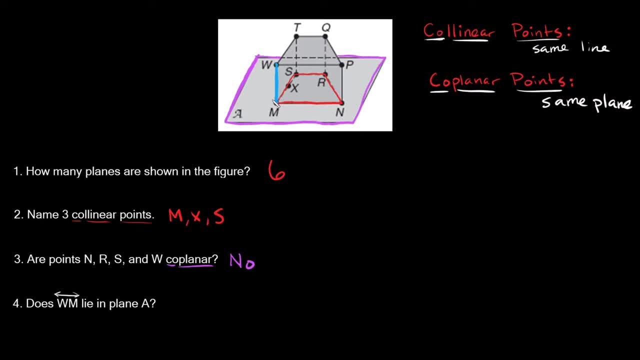 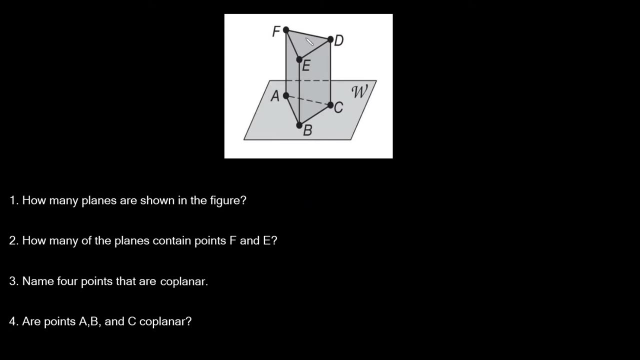 lying on the table. Okay, so this line right here, w m, does not lie on plane a. Okay, so number four would also be a hell. no, All right. here's our last problem, And this is the figure we're working with this time, Okay, which basically looks like a Toblerone, If you don't know what that. 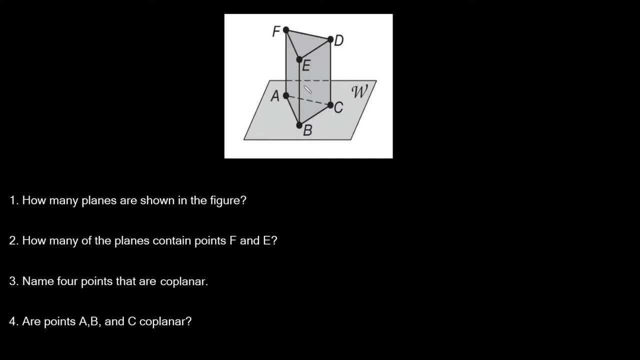 is go ahead and google it, But I guess technically this would be called a triangular prism, All right, so the first question asks how many planes are shown in the figure? Okay, so again, just count up the sides of the prism, aka the Toblerone, All right, so the first side that we're going to count. 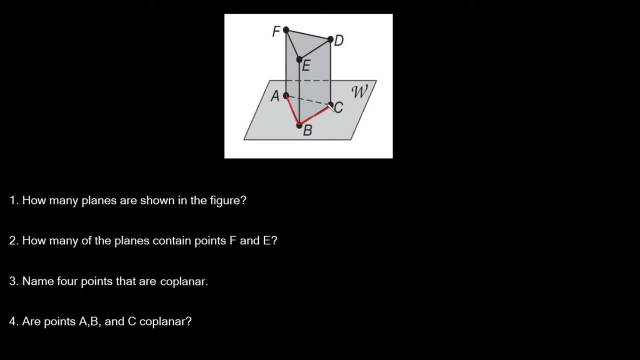 is this bottom side right here, a, b, c. Okay, that's the bottom part Right. that's the part that's touching the table over here w Right, plane w. So that's our first one. The second one would be this side here. Okay, this is one of the sides of our triangular prism, So that's number two, Okay. 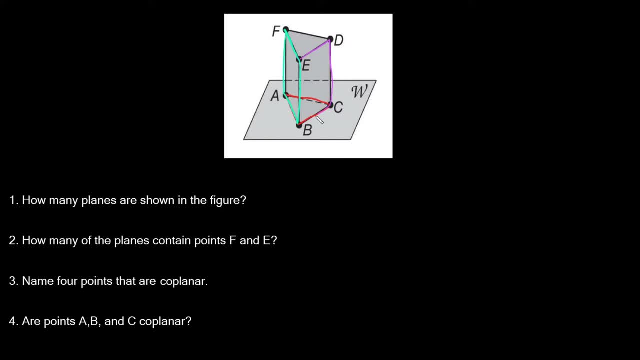 number three would be this other side right here on the right, So that's number three. And then we also have the back right, So this back part over here, that's number four, Okay. and lastly, we have the top, The top of our triangular prism, So number five, Okay. so how many planes do we have? 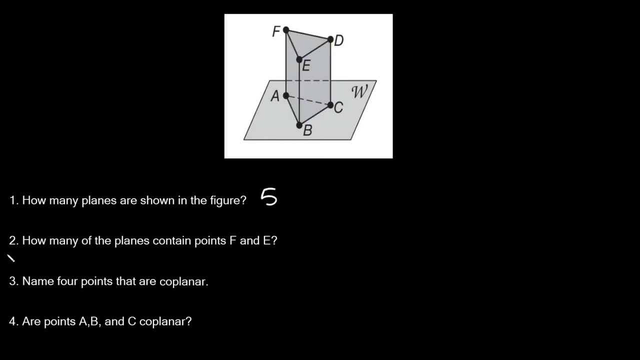 here We have five planes, All right. number two: How many of the planes contain points f and e? Okay, so, how many of the planes contain both of these points right here, f and e? Well, f and e are right here, Right so? 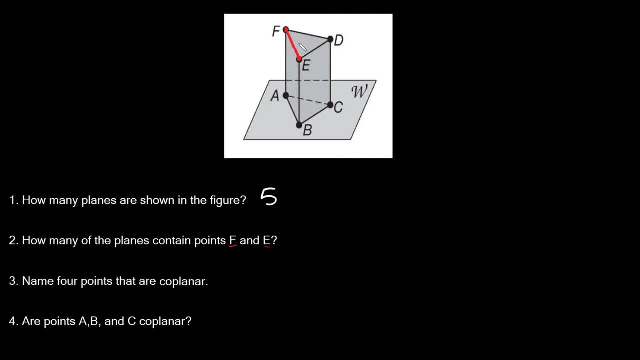 these two produce this line right here. Okay. so how many of the planes contain this line f e? Well, there's basically two Right, so there's this one right here, this side of the triangle- Okay, that contains f e. and also the top Right, the top part right here, also contains the line f e. Okay so 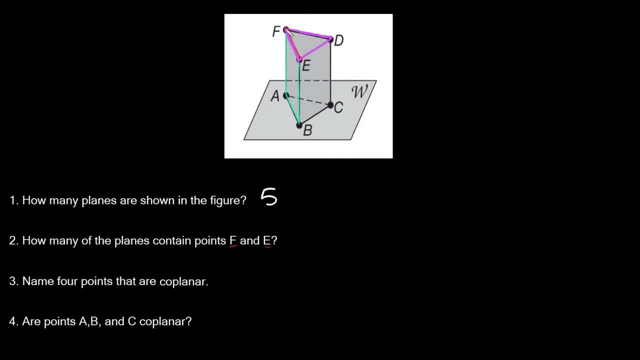 there's two planes, this blue one and this purple one, that contain f and e. Right, so number two would be a two, All right. number three: Name: four points that are co-planar. Okay, so this is a for four points that are on the same plane. okay, four points on the same plane. 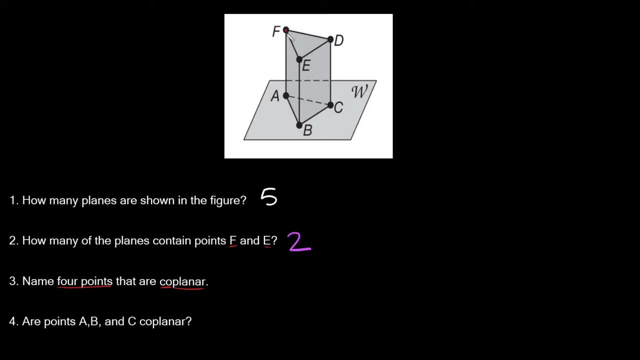 okay, so you basically have three options. so you can go F A, B, E, right there. you can also go E, B, C, D, right there. okay, that's four on that plane. or you could go with the back F A, C, D- okay, that plane also has four points. okay, so you could. 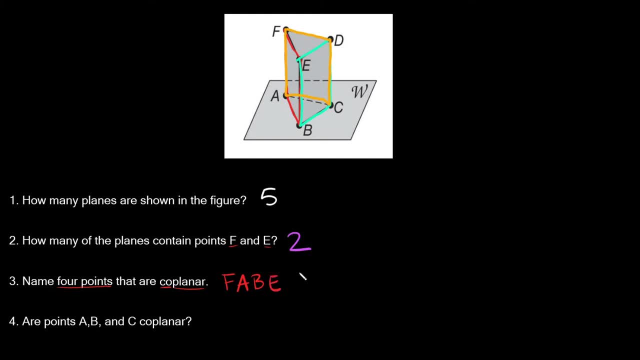 go again F A, B, E. you could go E, B, C, D, or you could go with the back one: F A, C, D. alright, you can use any of these for your answer, all right? lastly, number four, our points A, B and C: servir para aconsej jamar. 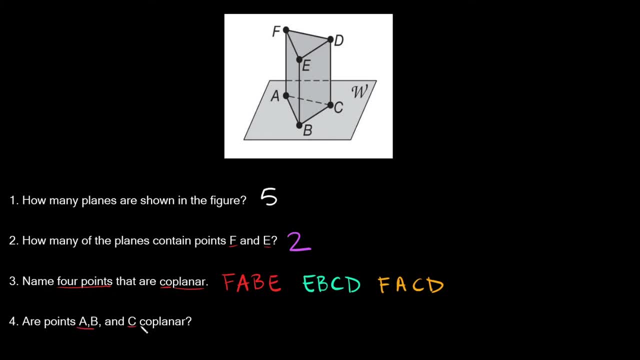 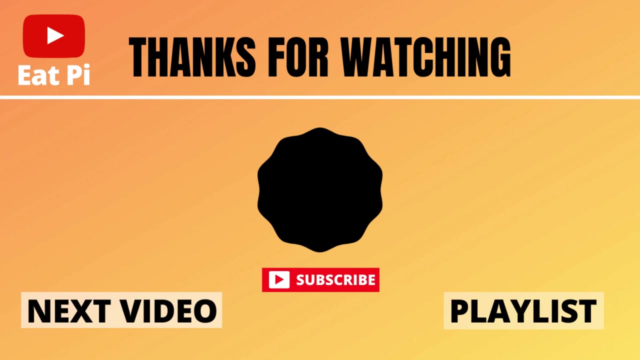 planar. okay, so our a, b and c on the same plane, all right? well, a, b and c are right there, right? and, as you can see, they're all on the same side of the triangle, right? so our a, b and c coplanar, hell yes. so if you found the video helpful, definitely leave a thumbs up down below. 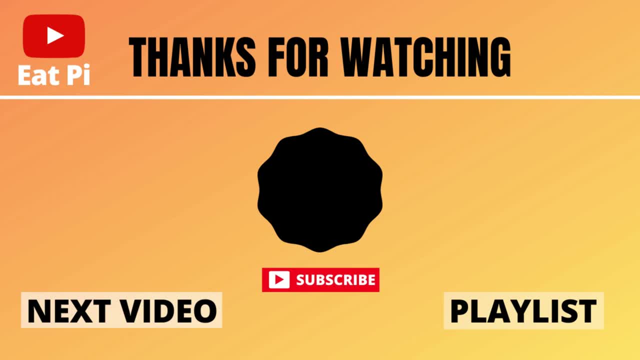 and if you have any other questions or want to see any other examples, just let me know. in the comment section below also, there's a couple playlists attached that i think you'll find helpful, so definitely check those out and i'll see you there.